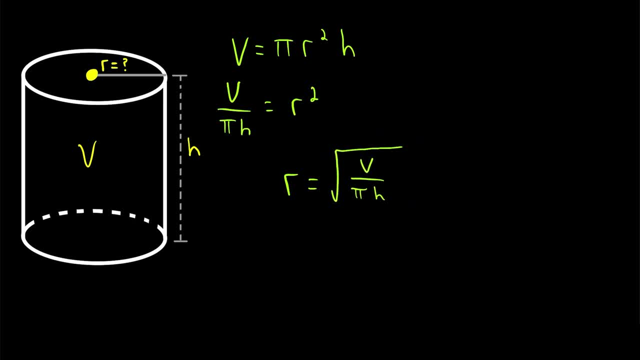 the radius on the left side of the equation, because that looks nicer. So it's as easy that if we want to find the radius of a cylinder and we're given the volume and the height, all we have to do is divide the volume by pi times height and then take the square root and that is our. 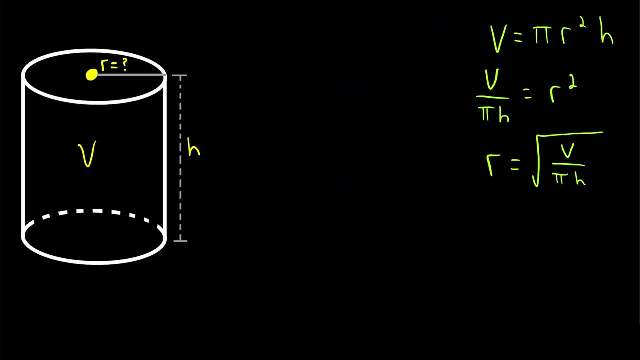 radius. so let's move this work to the side and check out an actual example. let's say it's given that the volume is 5 meters cubed and the height of our cylinder is, let's say, 2 meters. now, in order to find the radius, we could plug these values into this equation and solve for r again, or we. 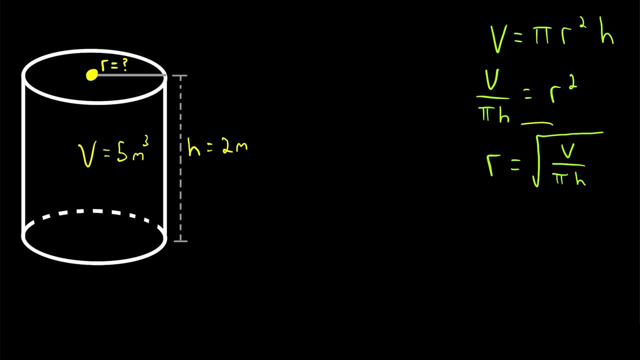 could just apply this equation that we just figured out. let's first just try applying this equation. so the radius is equal to the square root of the volume, which in this case is 5 meters cubed. so 5 meters cubed divided by pi times the height, in this case, that's pi times the height of. 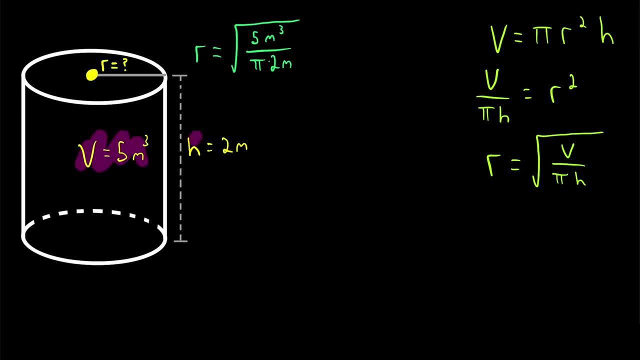 2 meters and that's going to give us 4 meters. now, as long as you're given the volume and the height in the same base unit, in this case meters, then it's not really necessary to work with the units when you're solving for the radius, because as long as we do everything right, the final 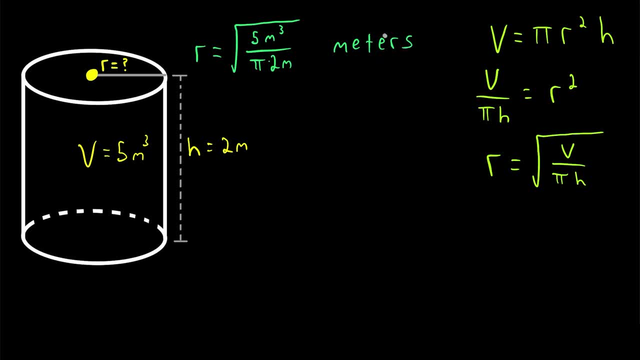 number is going to come out to be a number measured in meters, but i'm going to work with the units in this example, just to show you that, indeed, that is the case. our final number will be in meters. you would have to be a bit more careful, though, if, for example, your volume is 1.5 meters. 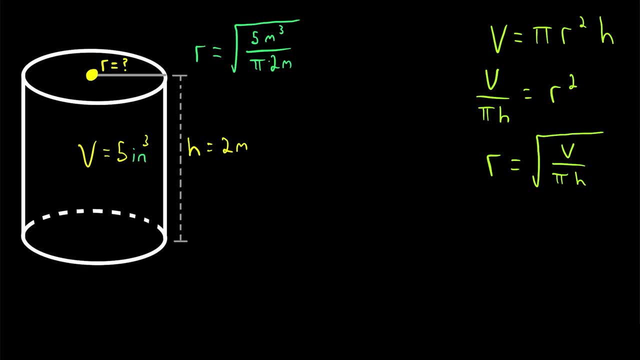 instead of 2.5 meters, volume was given in inches cubed and your height was given in meters. You'd have to choose to either convert to inches or convert the inches cubed to meters cubed, Or you could convert them both to something else entirely, like centimeters cubed and centimeters, but that would seem like. 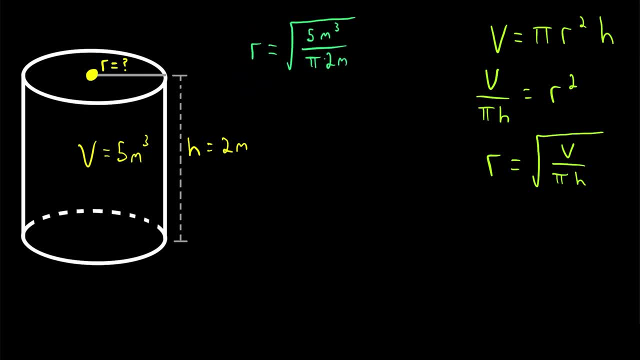 an unnecessary thing to do. All right, so let's go ahead and simplify this and we'll quickly find our radius. Notice that we've got meters cubed in the numerator and we've got meters in the denominator. Meters cubed divided by meters is meters squared, So we can rewrite this expression. 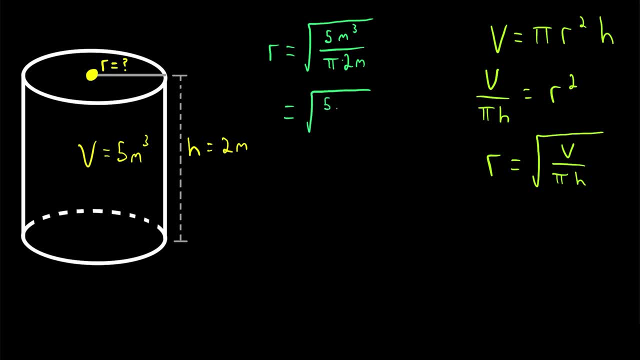 as the square root of 5 meters squared, divided by pi times 2, which I'll write as 2 pi. Again, all we did in that step was divide meters cubed by meters. That leaves us with meters squared. Now, since all we have under the square root is multiplication and division, we could take out: 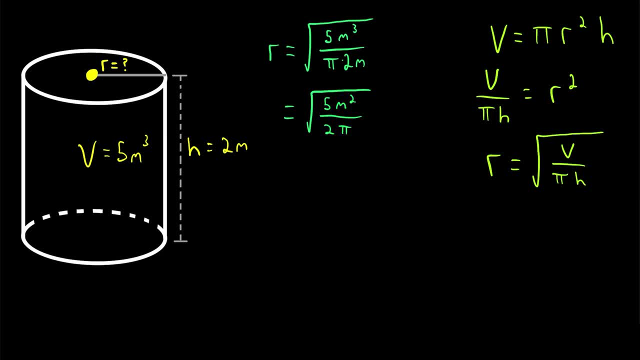 any of these factors and put them in their own square root. So we could rewrite it like this: the square root of 5 divided by 2 pi, and then taking out the meters squared, putting that under its own square root. The square root of meters squared, of course, is meters, which is why we 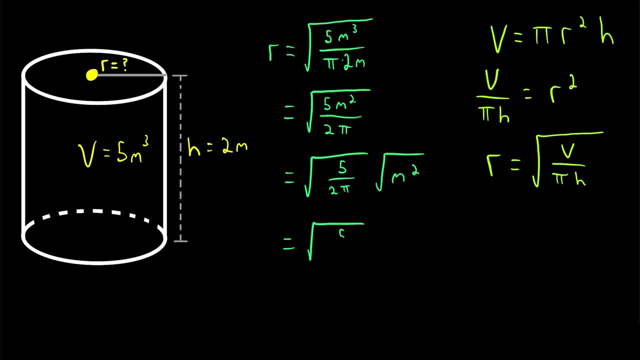 wanted to do that. So now we've got this simplified down to the square root of 5 divided by 2 pi meters. So we see that our radius is indeed in meters. as we would expect, We could leave our answer in this exact form, or we could approximate, If we approximate to. 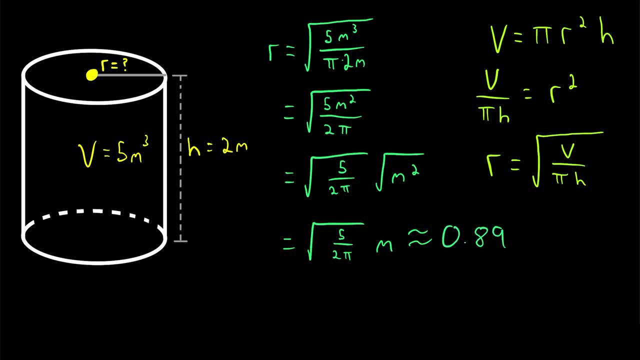 the nearest hundredth, this is about 0.89 meters, And so that is how we can apply the formula we found in order to find the radius of a cylinder when given the volume and the height. But frankly, this isn't quite how I would solve for the radius of a cylinder, So let's go ahead and do that. 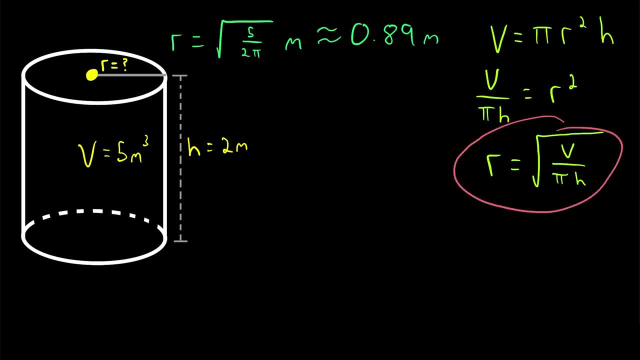 I think it's kind of unnecessary to remember another form of the same equation. So what I would do is just apply the volume equation I already know and I just solve for r again, because it doesn't take long. So I would just say: okay, we've got our volume of 5 meters cubed. 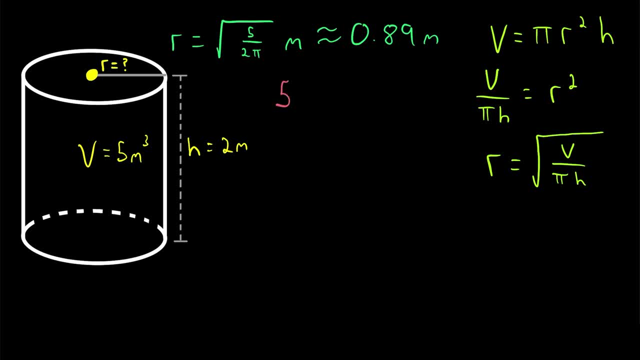 I know that the final unit is going to be meters, so I'm not even going to bother writing the units in this equation. So the volume is 5 meters cubed, and then on the right side of the equation we've got pi? r squared. I want to solve for r. 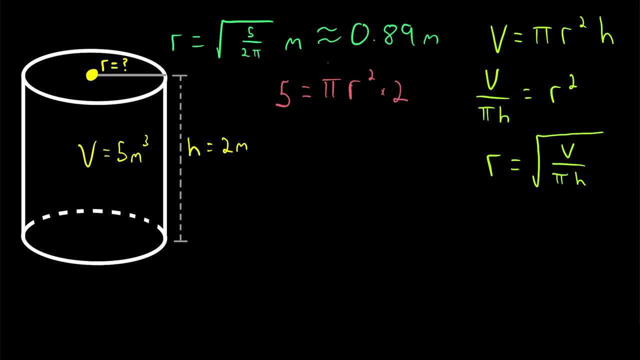 and then we've got the height, which is 2 meters. I'll just write that as 2.. Then I'll just divide both sides of the equation by 2 pi in order to get r squared by itself. And so we've got 5 divided. 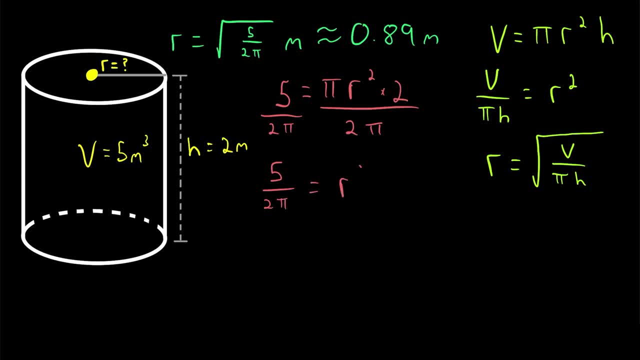 by 2 pi on the left side of the equation is equal to r squared. Then we just got to take the square root of both sides And again we have that the radius is equal to the square root of 5 divided by 2 pi. So very quickly we arrive at the same answer as before, but we didn't have to.